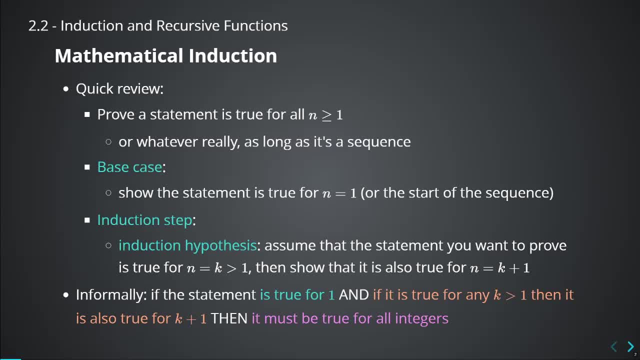 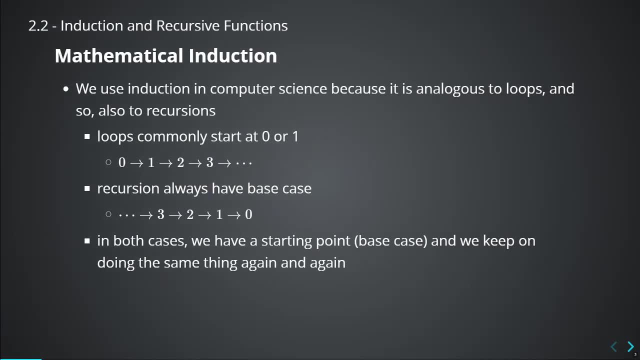 For all positive values of n, And that's what induction is. And so induction is very closely related to loops and also to recursions and computer science, Because that's pretty much what we do in loops and recursions: When you have a loop, you always start at 0 or 1.. Well, 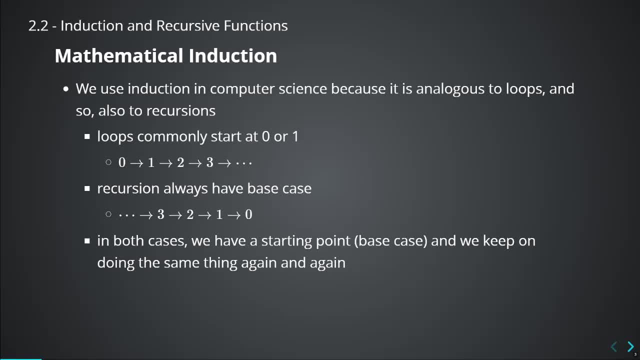 most of the time you will start at 0 or 1.. So your progression goes like 0,, 1,, 2,, 3, and so on. When you have a recursion, you will always have a base case. If it's a recursion that actually stops, you will have a base case. 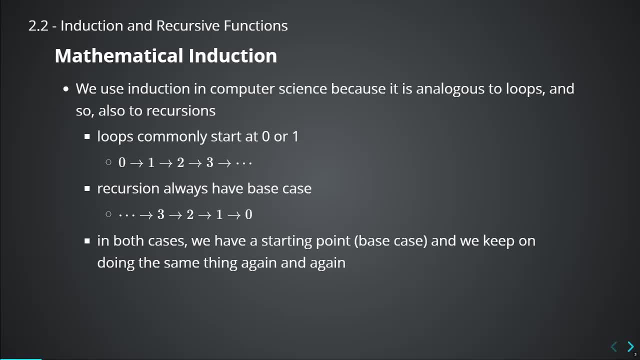 So it's the other way around. now. Let's say your base case is 0. Your recursion will go 3,, 2,, 1, and it goes to 0, and it stops. And in both recursion and loops we have a signing point. 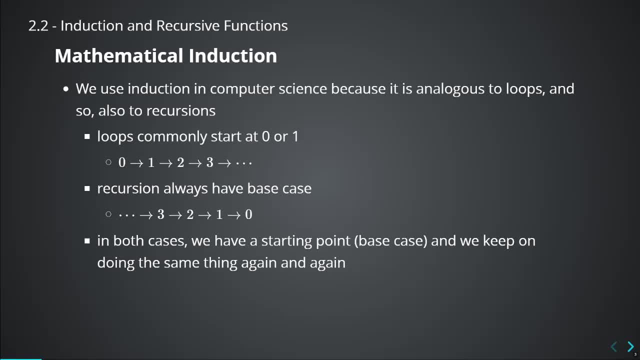 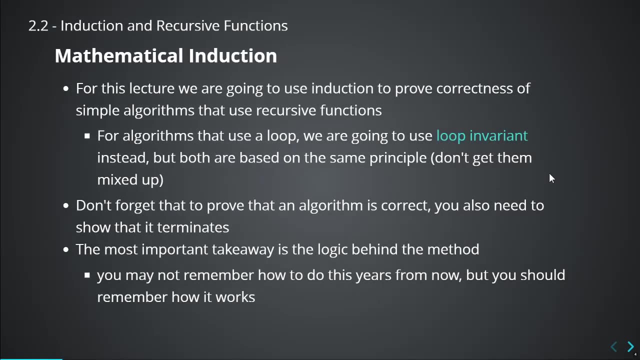 And we keep on doing the same thing again and again. So it's only natural that we can use induction to try to prove the correctness of these two well of recursion and loops. So for this lecture we're only going to be talking about algorithms that have 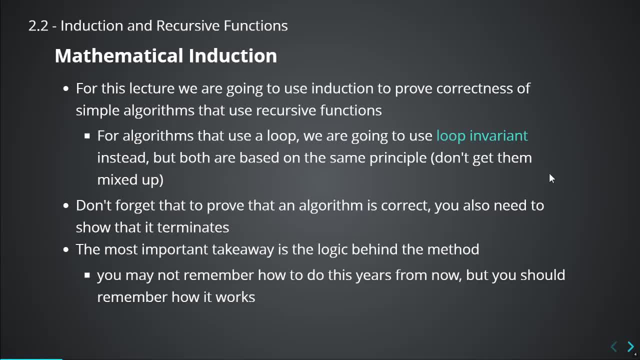 recursive functions in it. If you want to show the correctness of an algorithm that has a loop in it, then you have to use a loop variant. That's what we're going to be talking about in the next lecture. So both are based on the same principles. sure, But make sure you don't get them mixed up. 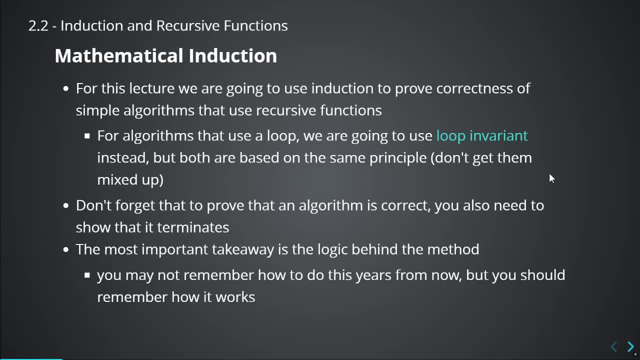 Because if I ask you a question to show something using a loop variant, like here, I'll give you a iterative algorithm And please use a looping variant to show that this is correct, And you have to use a loop variant to do that. People did get them mixed up last year. 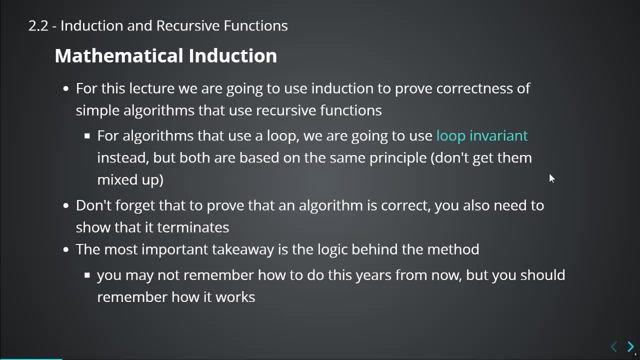 So please don't do that. Also, we're going to be doing simple algorithms only like stuff you already know how to write in first year and second year, because you are learning something new here, So we use something simple to show it to you. It's just like when you learn programming first time. 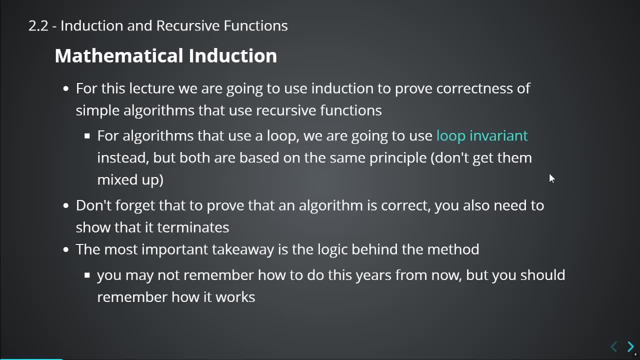 you'll be solving things easily. So we're going to show you how to do that, And then we're going to talk about things like the basic problem. So same thing here: you're gonna be learning to prove something properly And I'm going to be throwing simple problems at you. Also. another important 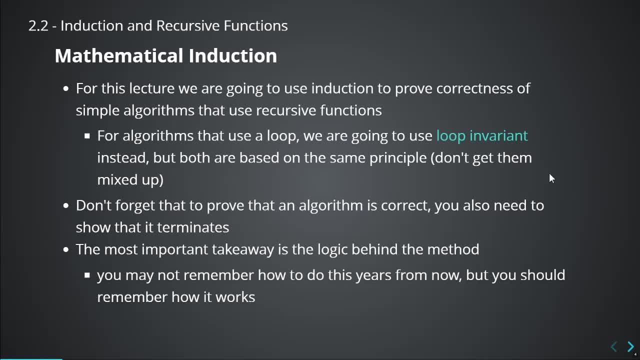 point there. don't forget that to show that an algorithm is correct, you have to show that at terminates. So sometimes that is an extra step that you have to take. But anyway, the most important takeaway from this lecture from this week, like all this talk about correctness, all. 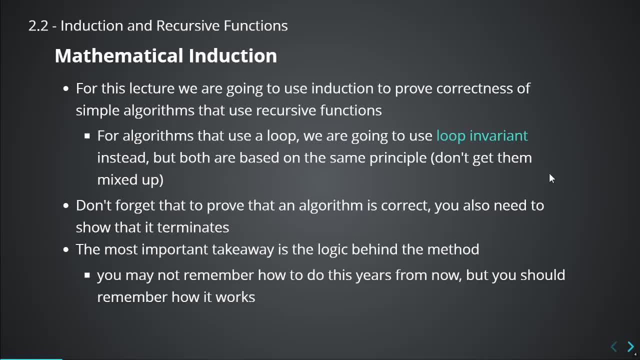 the stuff about proofing things. You may not remember how to do this- This is just gonna give from now- but at least you have an idea how it works, and I always claim that you already do this in your mind anyway, when you're writing a code, when you're writing a loop, when you're writing a recursive function. 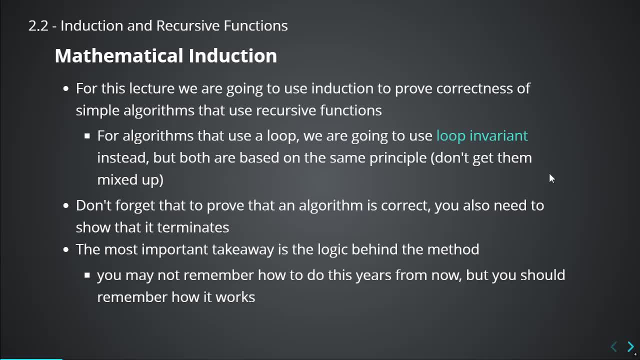 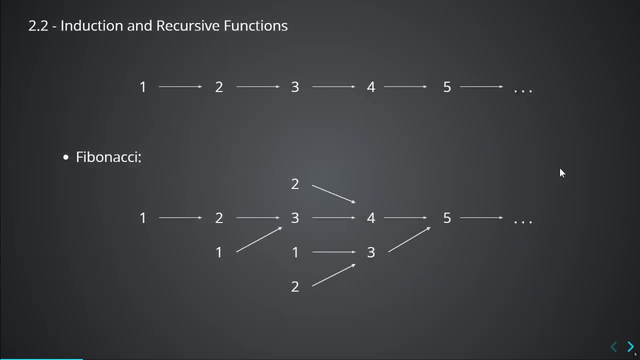 you already have an idea on how to write it correctly, so this whole idea of proving something is already in you, and we're just going to try to do that in writing formally with this unit. now, one thing that is slightly different from algorithms with recursive functions and just induction. 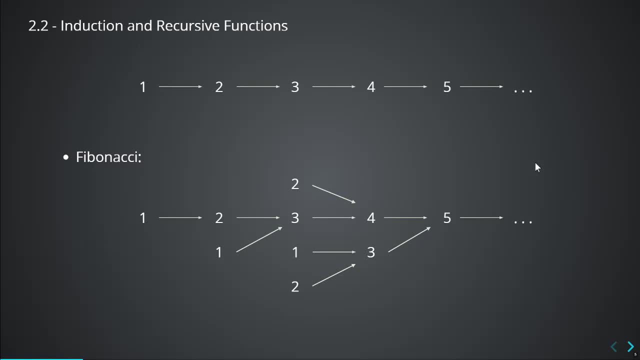 well, when you see induction, most of the time you only see a progression from 1 to 2, to 3 to 4. it's like a linear progression, just one case to the next case, to the next case, to the next case, and obviously that's not true. 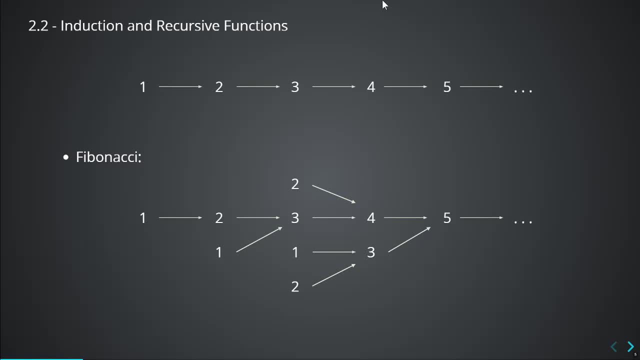 with recursive functions, at least once you've been writing. I mean, if you have Fibonacci- something very simple like a Fibonacci function- well, this is something you should not be writing in a recursive manner. but if you do write Fibonacci recursively, you can see that. 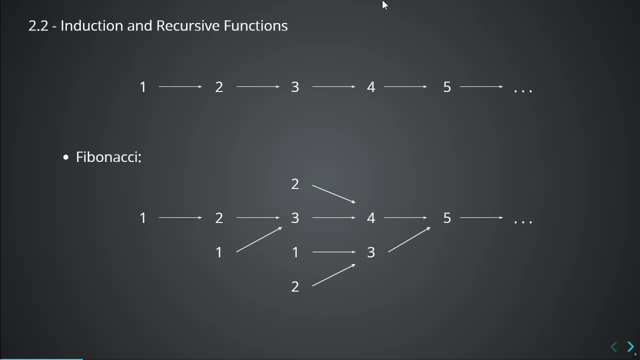 one case depends on two other cases. if you want to count Fibonacci 4,, you need to compute Fibonacci 3 and Fibonacci 2, so of course this makes analyzing the correctness much harder, because one case will spawn many, many cases, so we'll try to avoid those ones. 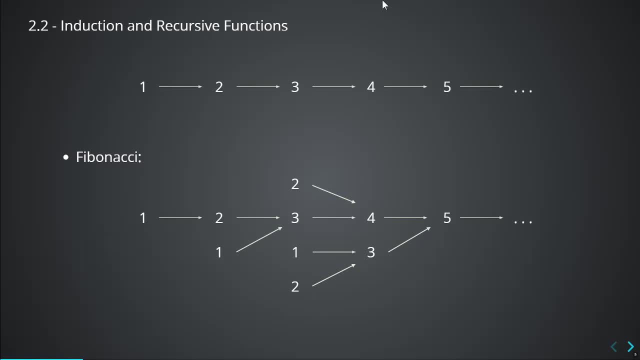 I do have one or two examples where you will have several cases and we can still do that, just like induction. actually, you can still use induction when you have several cases. but yeah, just be aware of this and we're going to start very simple, we're going to start very slow. 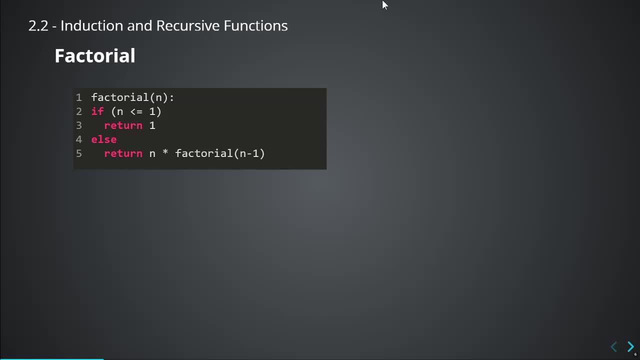 we're going to start with a function to compute factorial, and that's what we have done in the first year, I'm sure. in fact, this is the example that I used in the previous video when I talked about proof by induction, which is a bit silly because it's just a definition of factorial. 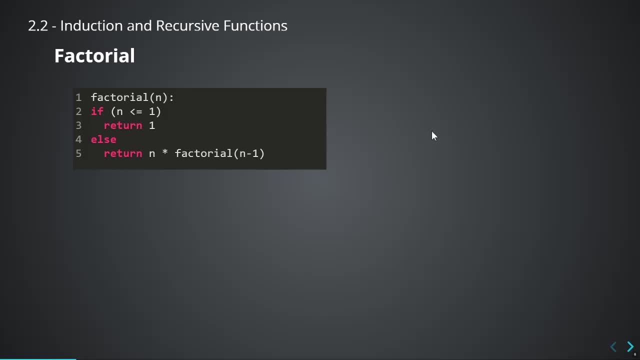 but if you want to, you can look at the previous video and check out the similarities between the proof by induction and what we're going to be doing now. so in both cases, we always start with the base case and we basically have to show that this algorithm is correct. 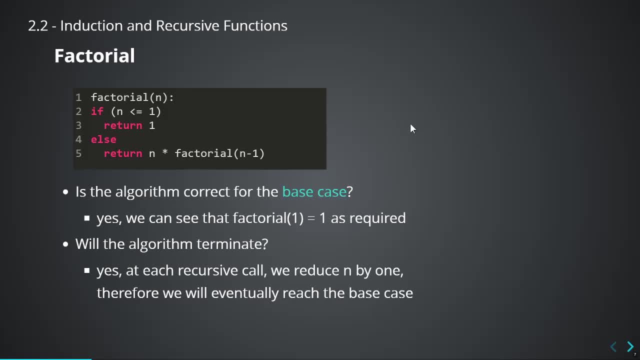 and n is equal to one. that's the base case there. and yes, it is, because factorial one is just one. that's the definition of one factorial. so, yes, the algorithm is correct for the base case. now will the algorithm terminate? yes, because every time you call this function recursively. 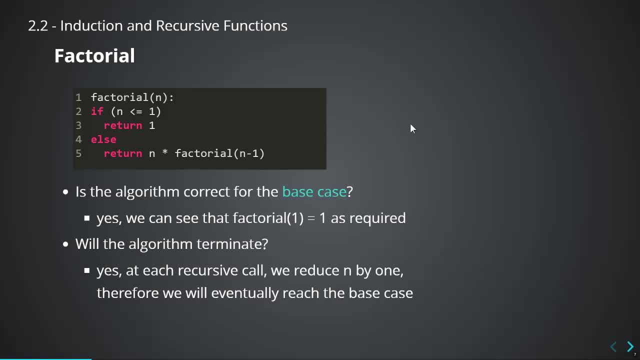 you reduce n by one, so eventually n will hit one. if n is greater than one, eventually it will be reduced down to one. if n is already less than one, it will just return one and finish the function call. so yes, it will terminate. next we go to the induction step. 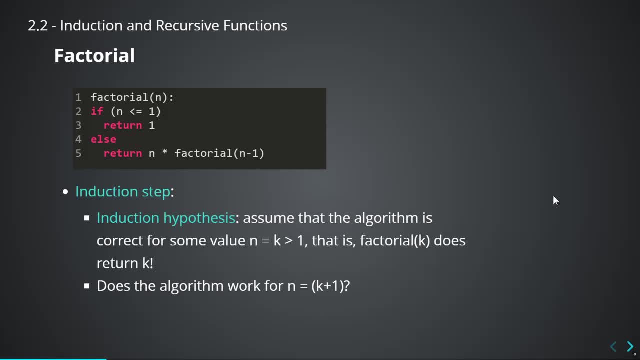 and our hypothesis here is that the algorithm is correct for some value k greater than one. so that means that we assume that factorial k does return k factorial. so we don't know if this is true, but we just assume that it is. so what we have to do now is we have to show that the algorithm is also correct for k plus one. 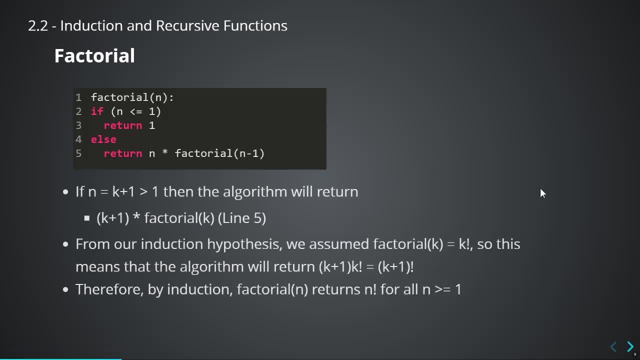 and this is where we have to do the most work. now, what happens when n is equal to k plus one? so we're going to be going to line five where we compute k plus one times factorial k. now we assume that factorial k is going to give us k factorial. 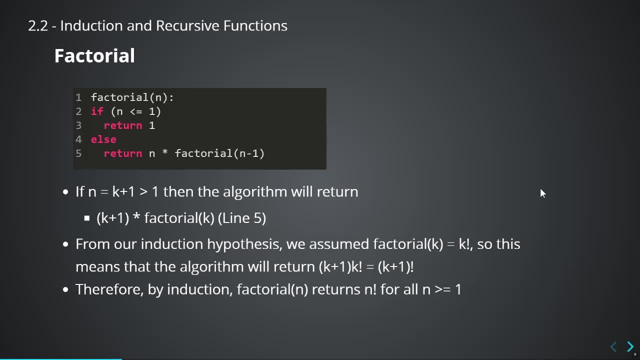 so line five is going to give us k plus one times k factorial, and that is the definition of k plus one factorial. so yeah, if the algorithm is correct for k, it will also be correct for k plus one. and there you have it. I have proved by induction. 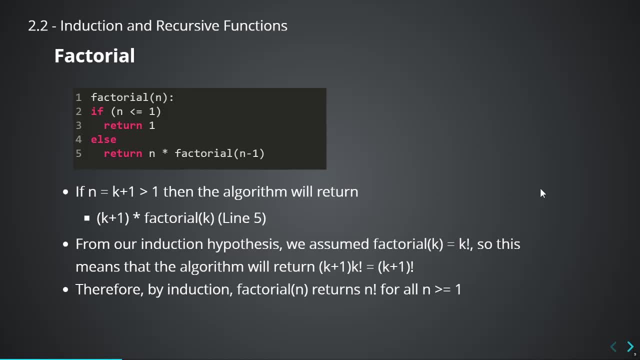 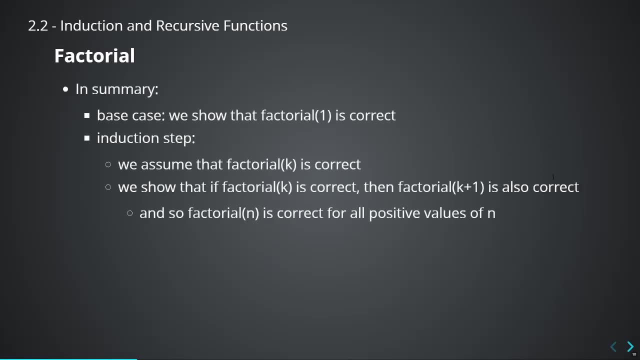 that factorial n returns n factorial for all n greater than or equal to one. so in summary, here's what happens: we show the base case, we show that factorial one is correct and then, with the induction step, we assume that factorial k is correct. and if k is correct, 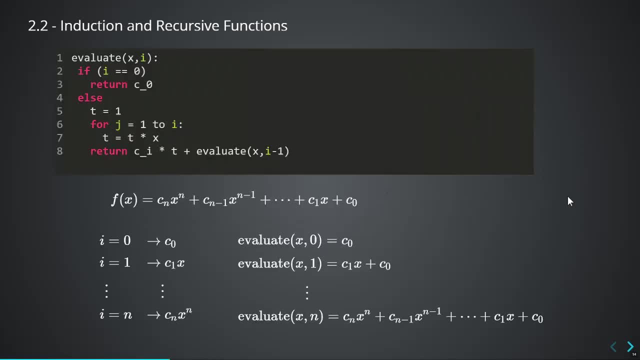 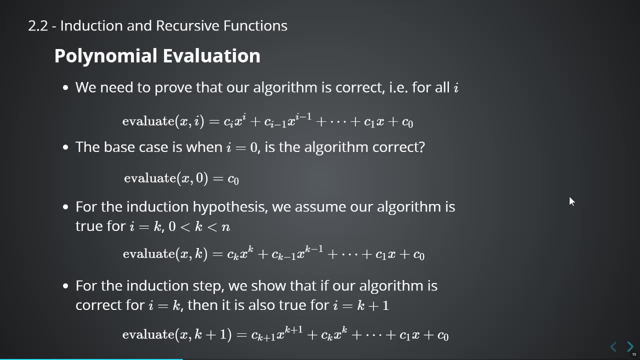 we show that factorial k plus one is also correct, and we're also going to use induction to show that this code is correct. specifically, we're going to show that this statement, the one that I'm highlighting now, is always true for different values of i, and I'm going to talk more about what value i can take in a bit. 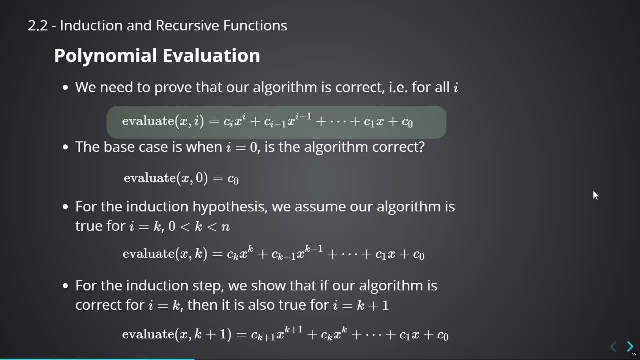 but we're going to be doing all the same thing. we're going to start from i equal to zero. we're going to show that the base case is correct. we're going to pick an induction hypothesis and then we're going to show that if this hypothesis 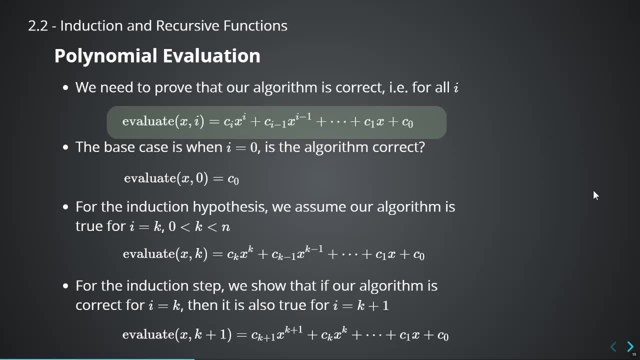 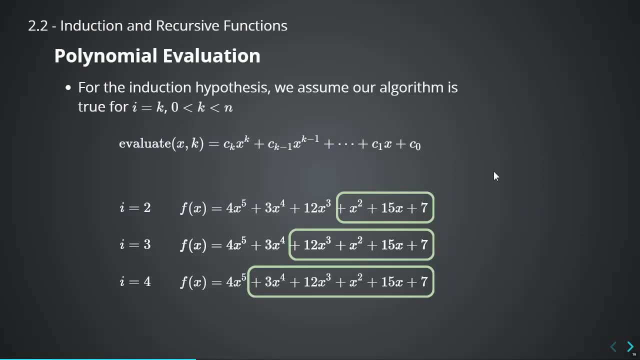 sorry. if it's correct for i equal to k, then we'll also show that the algorithm is correct for i: equal to k plus one. but just to be clear on how the algorithm works, just remember that we're computing the terms from the back. so if I give you, i equal to zero. 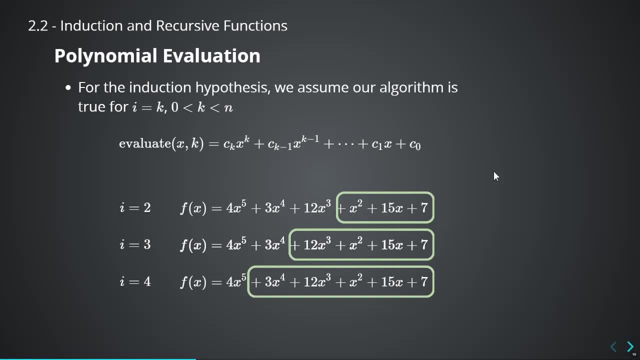 you're going to be giving me just the constant term. if I give you i equal to two, you're going to give me the last three terms. if you give me i equal to four, you're going to give me the final five terms. but the main goal here again, 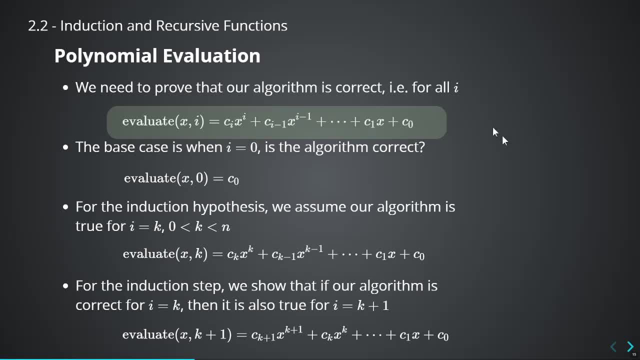 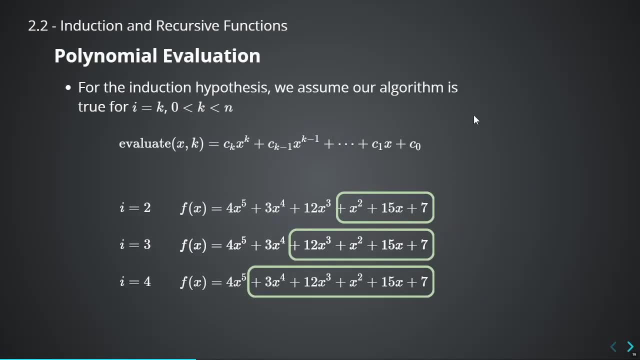 is to show that this statement, the one that I'm highlighting. we're going to show that this statement is always true for various values of i. now it's important to talk about what value i can take. obviously, this algorithm is not going to work if it exceeds n. 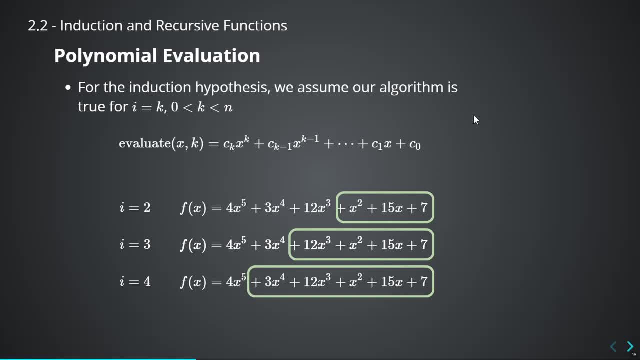 if you have a polynomial of degree n and then you give it n plus one, you've got a polynomial of degree ten and you give me i equal to twenty, then I won't be able to evaluate that. I mean, I can probably fix the code that handles that. 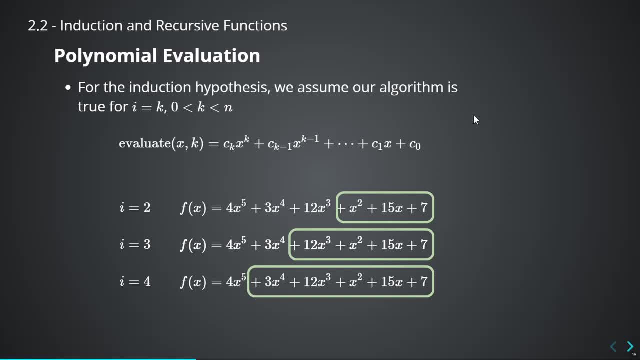 but let's just assume we're getting nice inputs. so for my induction hypothesis, I assume that the statement is correct for k, for i, equal to k is going to be between zero and n, so greater than zero and less than n. and while we're on that topic, 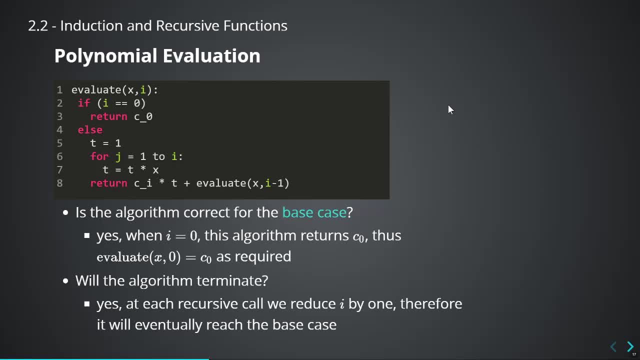 I should probably do something about the i on this function as well. on line two, because what happens if someone gives i equal to negative five, for example? that will screw up the code. so let's just assume that the input is going to be nice, that someone's going to give you i between zero. 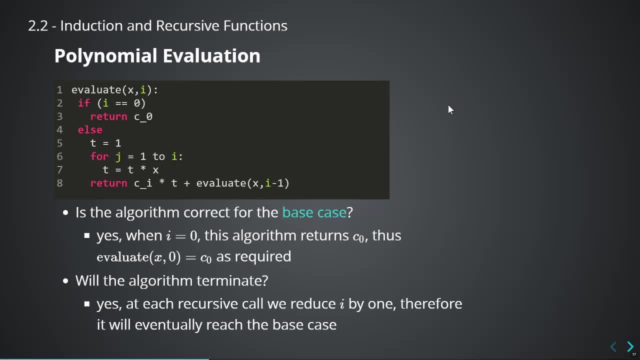 and n all the time because I just want to focus on how to do the induction. um, we can take care of all these little um problems, like you, just modify the code a bit more. but if I do that, I'm just going to over complicate the code. 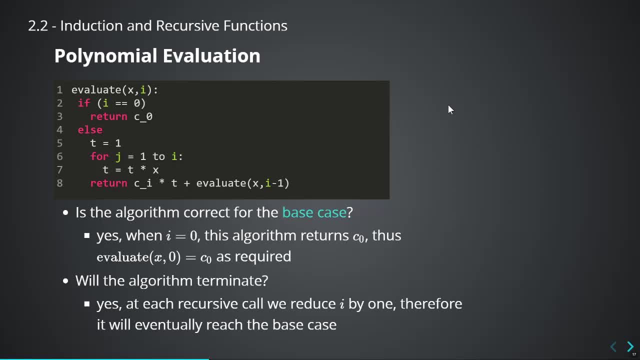 so I think it's just better to just mention that I do have some problems here. it's not completely theirs, but the focus is on how we do the induction, so just keep that in mind. alright, now the base case is the statement correct when i equal to zero. 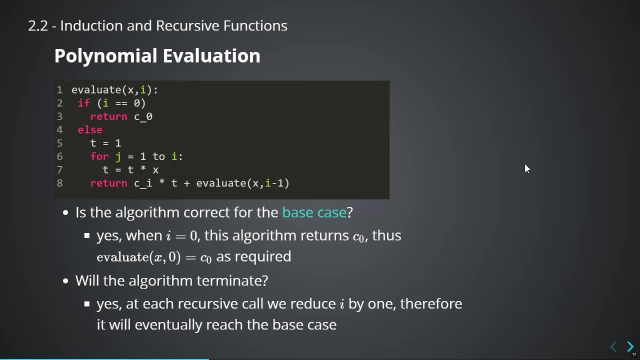 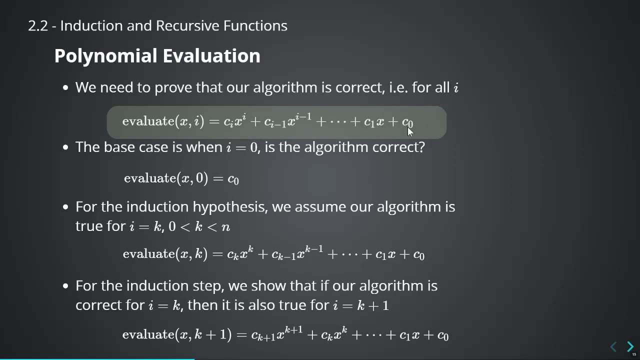 well, when i equal to zero, I just want to return the constant terms. and when i equal to zero, the statement does return just c, zero, right, when i equal to zero, everything else will be zero. so just kind of return the constant term. so, yeah, the statement, the function evaluate. 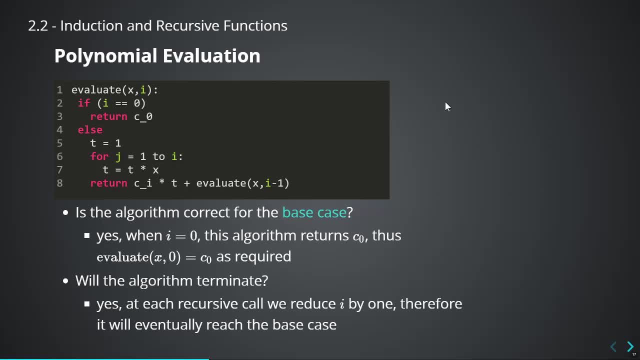 x zero is correct. it gives me c zero. will the algorithm terminate? uh, yeah, it will, because, um, if you give me a positive i, I'm going to recurse and I'm going to reduce i by one every time I recurse. so eventually it will reach the base case. it will eventually reach i equal to zero. 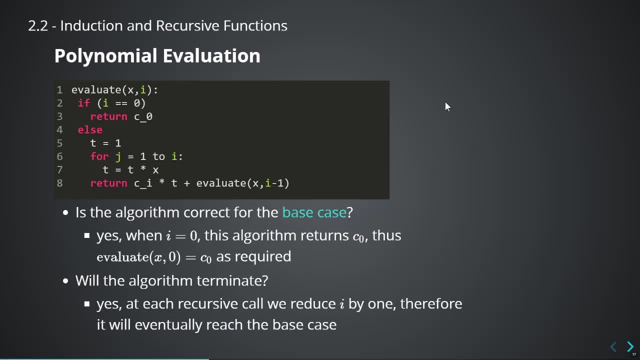 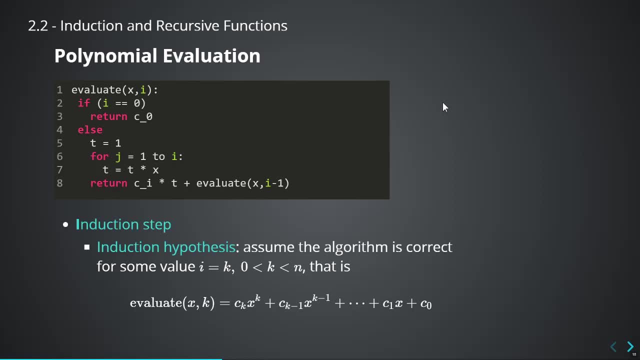 and, yes, it will terminate. okay for the induction step. well, the induction hypothesis is just the same statement, again with um i equal to k and, as I mentioned, I'm going to say that um k must be greater than zero and must be less than n. so pretty simple there. and what we 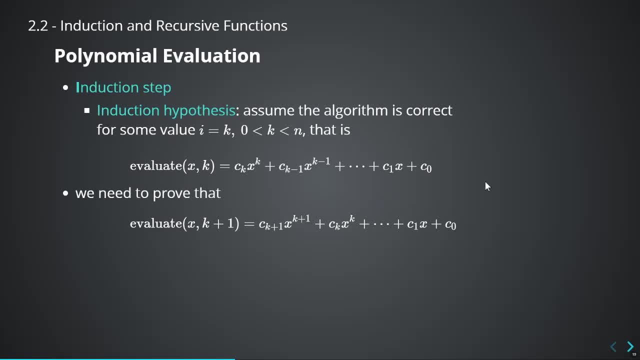 have to do is we have to show that, assuming the um evaluate k- sorry, evaluate x k- is correct, then evaluate x k plus one will also be correct, as in: it will give me uh c k plus one times x to the k plus one plus c k, x to the k plus. 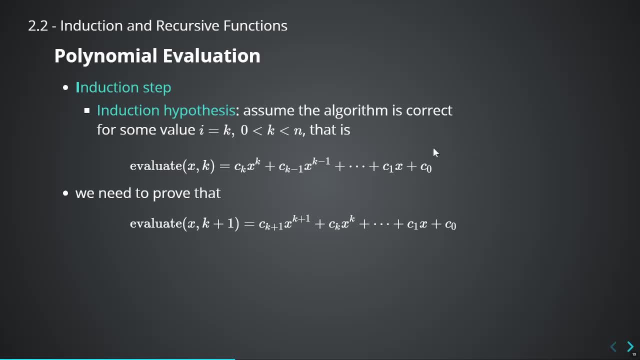 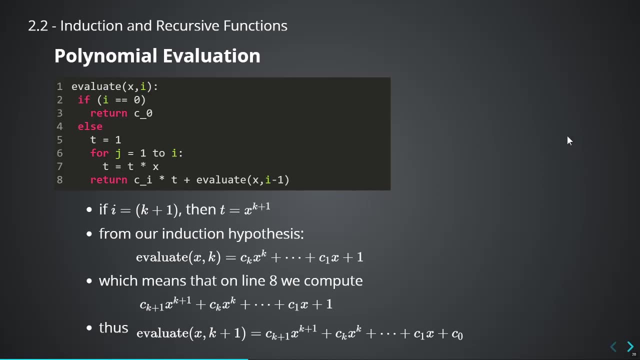 dot, dot, dot plus one. yeah, so how do we do that? well, let's look at the code. when i is equal to k plus one, then the loop from line five to line seven is going to compute uh, x to the k plus one. that's what t is. 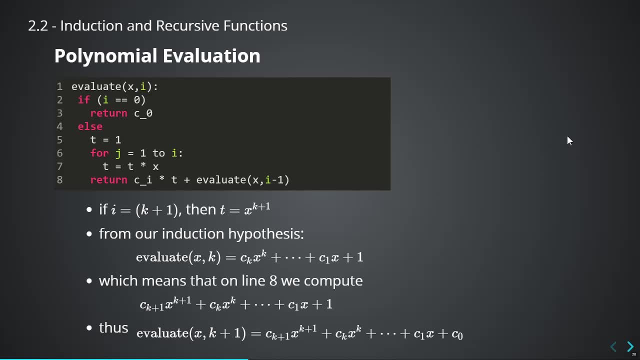 going to be now. from our induction hypothesis, we assume that evaluate x, k is going to give me c, k, x to the k plus dot dot dot plus c, one x plus one. so all we're doing in line eight, which is um, computing c, k plus one times t. 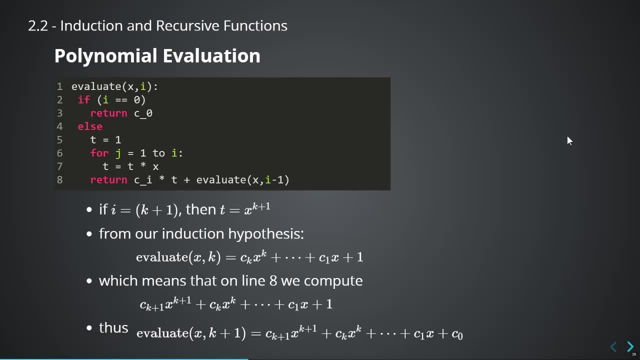 which is c, k plus one times x to the k plus one, and we add the written value of evaluate x, k. so we just get the c, k, x to the k, uh plus dot, dot, dot, like the remaining term. sorry, this is pretty hard to read. i mean, i hope you can. 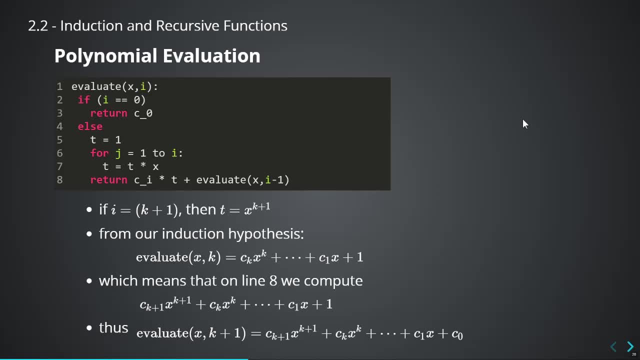 just follow from the my slides, because it's pretty hard for me to just read the polynomials like that. but then the point is we each have shown that evaluate x, k plus one does indeed give us c k plus one times x to the k plus one plus dot, dot, dot. 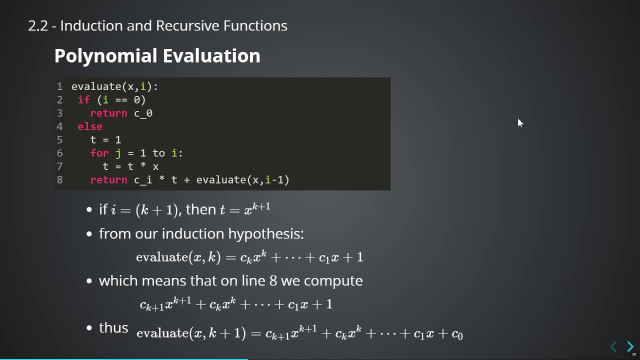 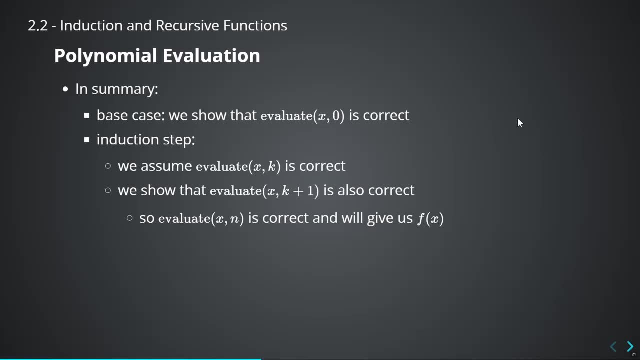 up to c zero, so the statement is correct. so, in summary, what we've done: we've got a statement. we want to prove um. we show that this statement is correct when um i equal to zero. so the function evaluate x- zero is correct. and then we go to. 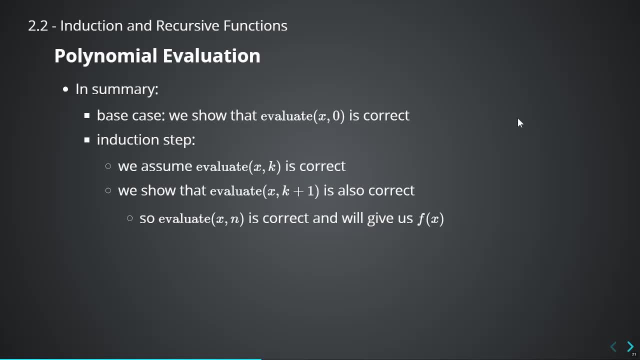 induction step. we assume that the function evaluate x- k is correct and then we show that if that is correct, then evaluate x- k plus one is also correct. so that means that evaluate x zero is correct, evaluate x one is correct, evaluate x two is correct and, more importantly, evaluate x. 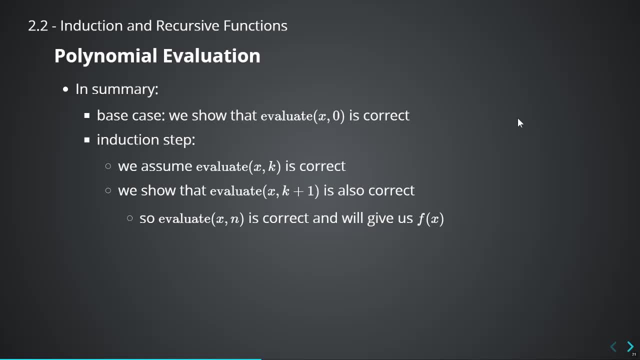 n is correct and it's going to give us f, x. so we're not going to say that this function is correct for all values of all possible values of n, well as in we're not going to say that evaluate x, i works for every possible value of i, because there's the limit on what 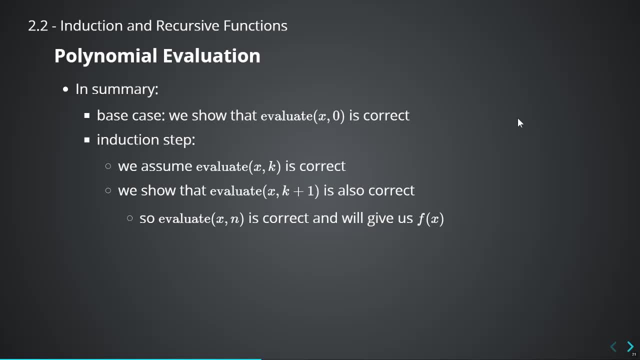 what value you can choose. right, because you have a polynomial of degree n. so you should use um input n in there, and if that's the input, it will work. it will give you the evaluation of f x. so that's the end of the proof, if very similar to the first one. 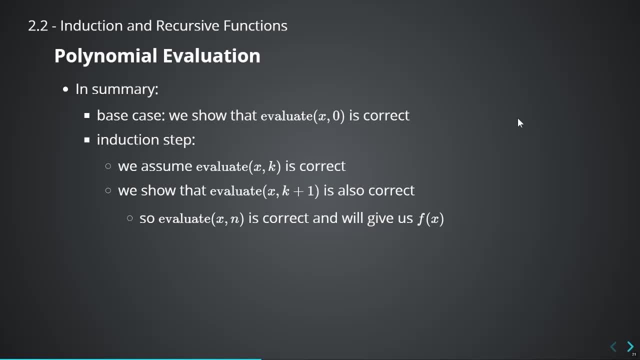 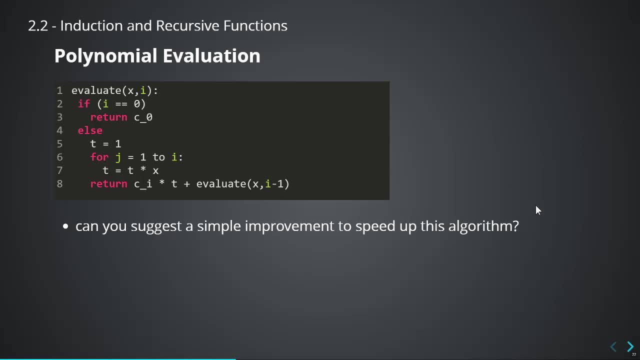 um, so i hope you can see that this is pretty straightforward, okay, so now let's go talk about complexity for a bit. let's go back to the code. i mentioned that this code is slow and i was wondering if you can suggest a simple improvement so that i can. 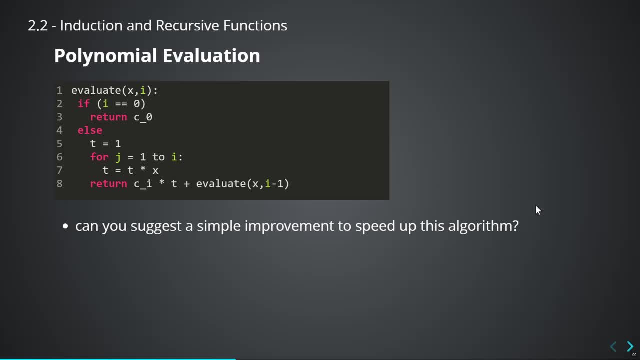 speed up this algorithm. so the reason why this code is slow is because every time i go to the function, every time i recurs, i have a for loop in there that will compute the powers of x. so i'm if i compute x to the 5, i have to multiple x 5. 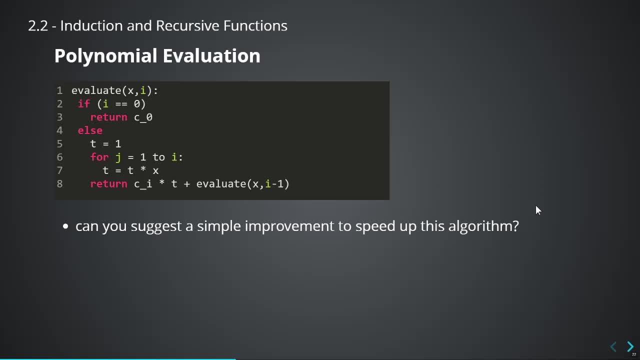 times. and then i come in the game and i go to 10, i have to compute x to the 10, i have to do the multiplication 10 times. so yeah, you can do the multiplication faster than just doing it. uh, like that. but you can also do this. 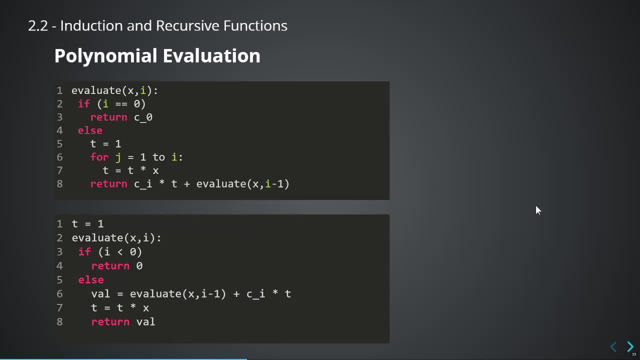 like. look at the second code. here i'm saying that every time you call the function uh, multiply t by x. so i'm gonna keep t as a global variable. then every time i come in the function, i increment t, i multiply by x. so yeah, it cost me one global variable. 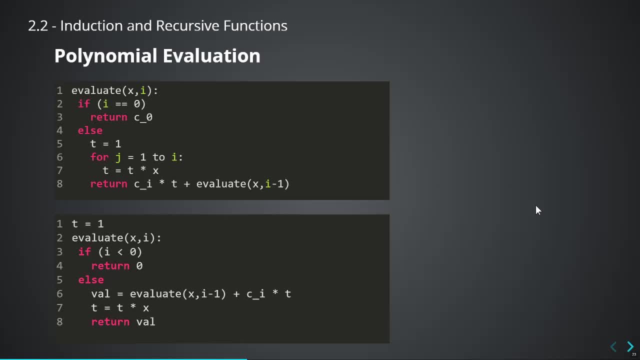 space. but now, every time i go inside the function, i just have to do one multiplication instead of doing a for loop. um, and i can actually do better. i can get from two multiplication to just one multiplication, and this is what we call the horner's method. 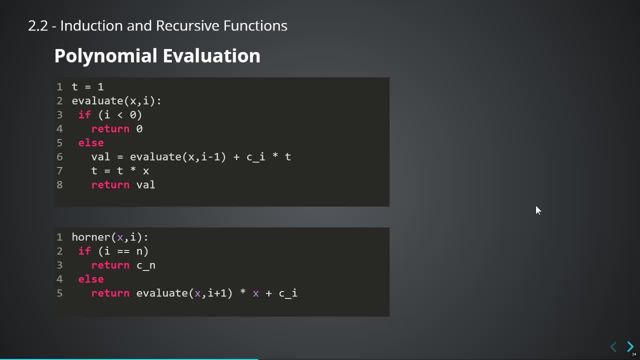 so this is pretty, um, uh, advanced code. um, well, it might be hard for some of you to understand, so we're going to talk about this code. um, you know, just feel free to pause the video and just run the code with some examples if you need to. 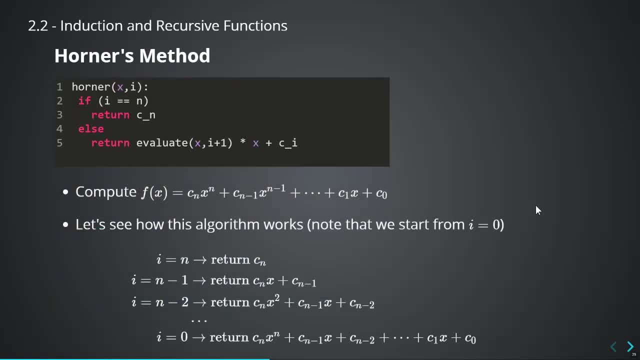 we're going to talk about horner's method. it's still the same thing. it's still going to compute the polynomial, it's going to evaluate the polynomial, but it works in a different way. now that we're going to start from zero, we're not going to start from. 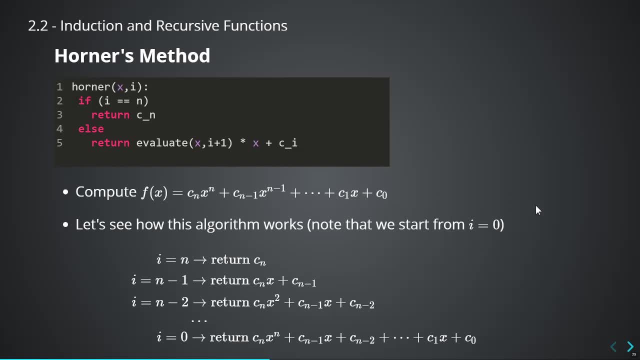 n. we're actually going to finish at n. when i is equal to n, that's when we finish. so when you call this, you have to call it from zero. so just think about what's happening when i is equal to n, when i is equal to n minus one. 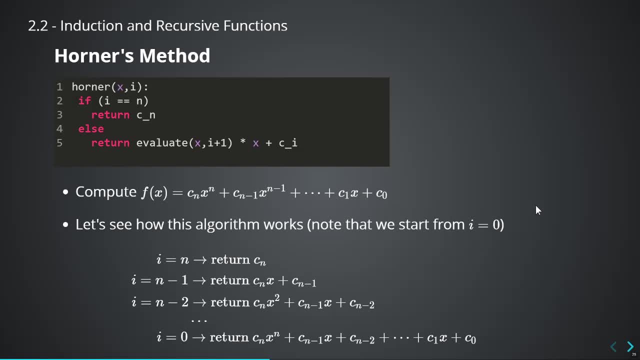 so on. right, so i have down there. so i'm going to call from i to zero. okay, we're just going to recur and calling um i equal to one, which is going to recur again, calling i equal um to two and so on. so you will um. 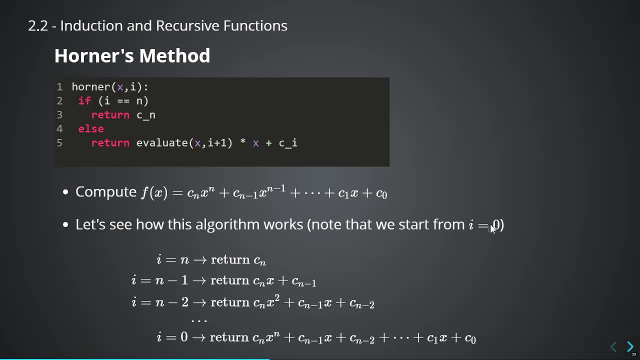 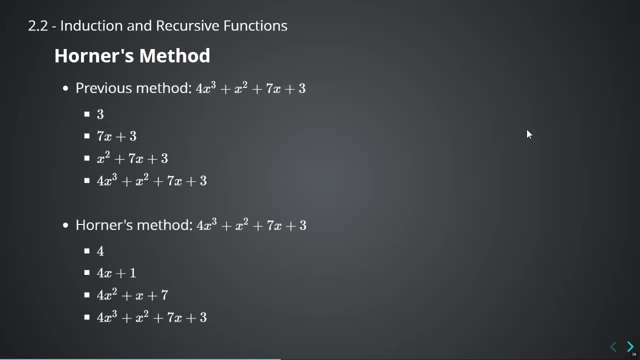 you will construct the polynomial in a strange way and like the other way around. i'll show you what i mean. like previously, uh, when you construct this polynomial, let's say four x cubed plus x squared, plus seven x plus three, right, you construct it from the constant. 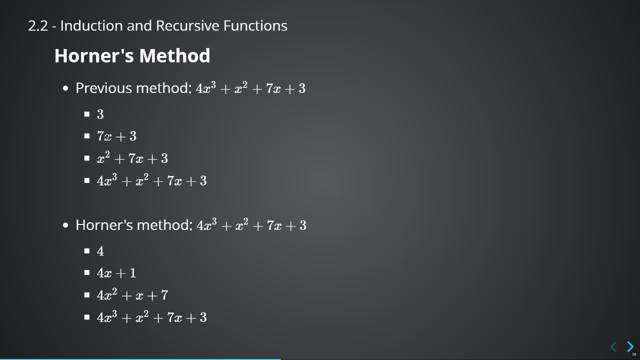 right, and then you work out the next um term, seven x, and you work out x squared and finally you will get four x cubed simple. with the honest method. you valid the same polynomial, you start from four and you're actually going to just compute four, right? and then you multiply that by 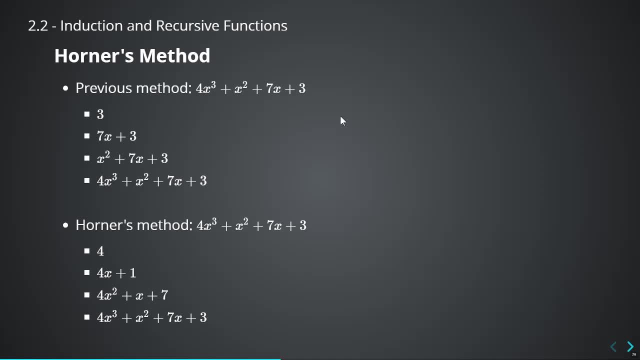 x and you add the next constant. so here the next constant is one. so i'm going to do four x plus one. you see, like four x plus one is not in the polynomial, like these are two terms which are not in the polynomial, you don't see four x. 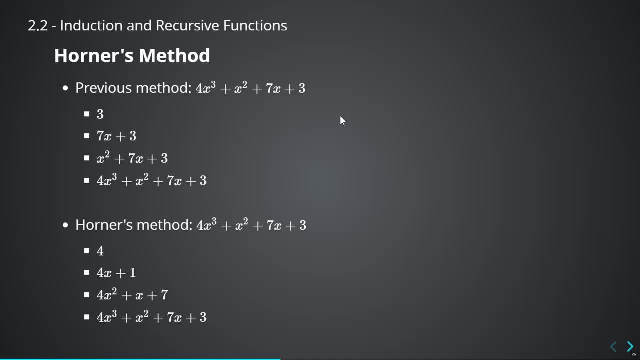 plus one. in there you see four x cube plus x squared. but this method works because, whatever, if you keep on multiplying by x, right um? next step, i'm gonna get four x squared plus x plus seven. it's getting there. and finally i'm gonna multiply by x again. 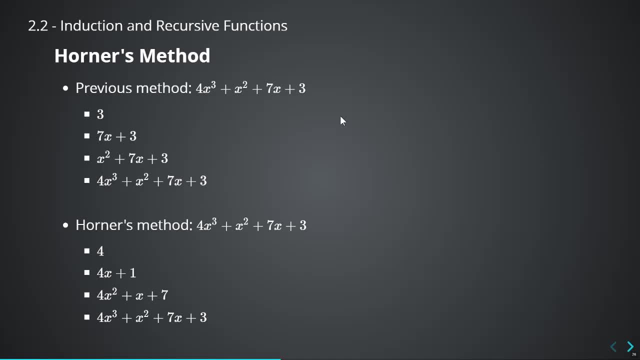 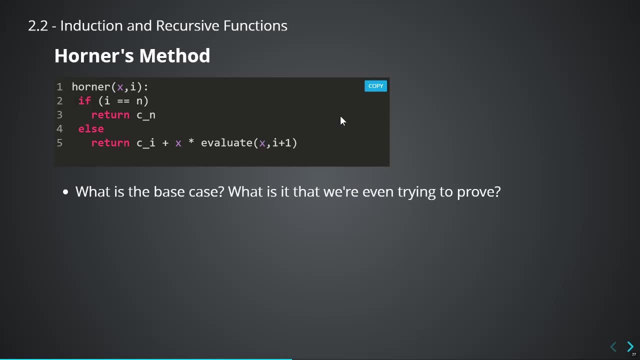 i'm gonna add three. i'm gonna get four x cube plus x squared plus seven x plus three. so this is the honest method and this is actually hard to evaluate. well, induction is always simple because in the induction you always do base case um, pick the uh. 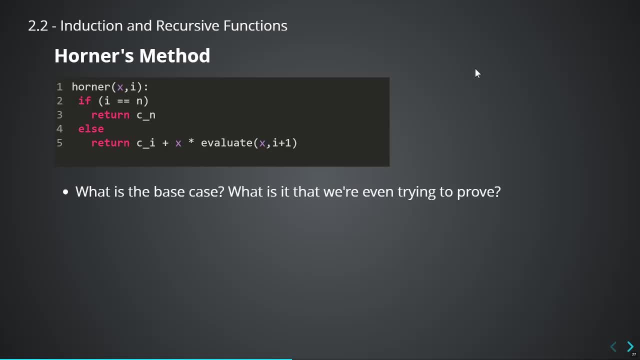 hypothesis, which is the statement you're trying to prove, um, and then you know if it's true for k. sure, that's true for k plus one. but now, what is the base case like even what? what are we even trying to prove? what is the statement that we're trying to? 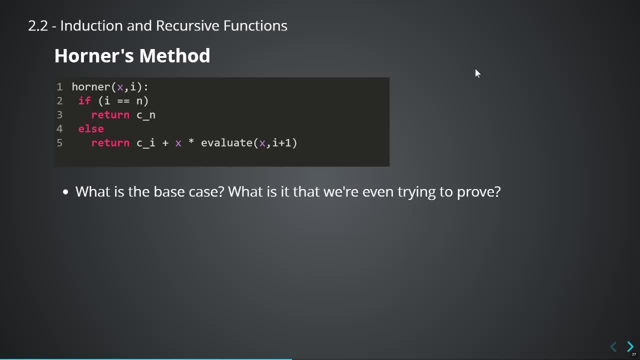 prove. the hard thing in this example is actually working out. what is it that we're trying to prove? what is the statement that we're trying to prove? so if you look at how the algorithm works, um, horner x- n is just c n, horner x- zero. 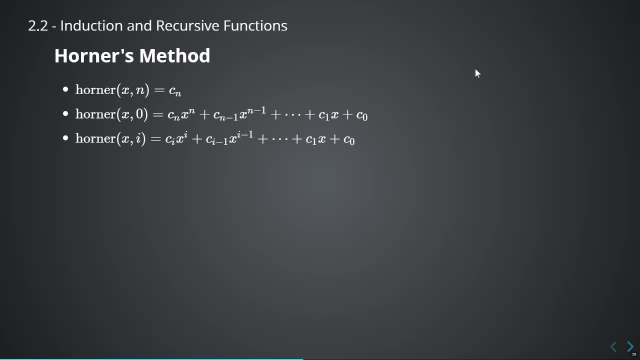 is actually the whole polynomial. that's the answer. so we start with um, we start with zero, but it goes back all the way up to n. so horner x- n will give you c n, horner x- zero will give you the whole polynomial. and i'm thinking: 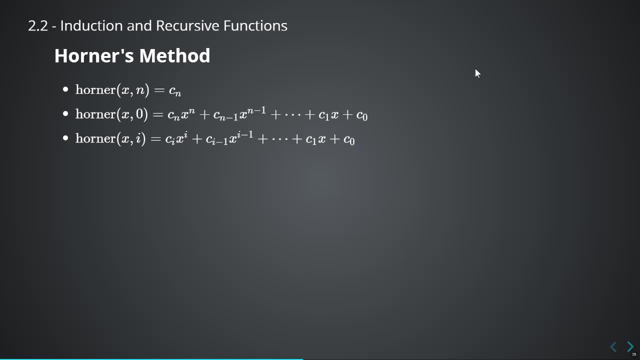 maybe i should say: horner x- i equal to c i x- i, plus whatever i have there, is it? well, actually not. this is the relationship, this is the. this is the statement we're trying to prove. so notice the uh subscript and superscript right. it's not c i x to the i. 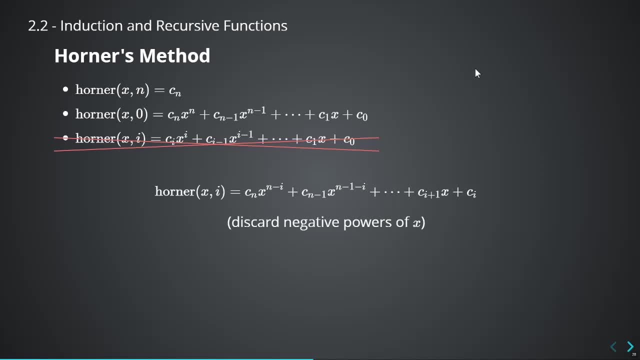 but it's actually c n times x to the n minus i, and we're just gonna discard negative house effect. so so imagine, if you put an n in there, if you put i equal to n, you're gonna have c n x to the n plus c n minus one times x to the. 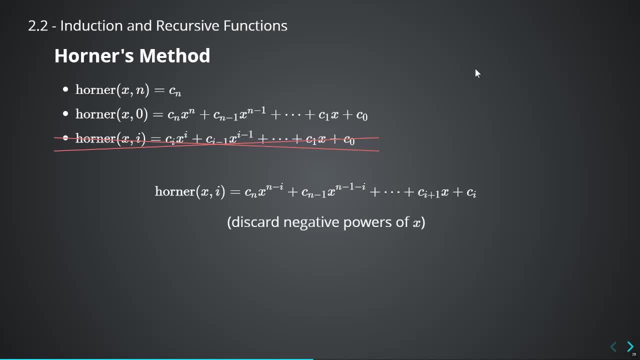 n minus one minus n, which is just x to the minus one. so we discard those, just just get rid of our negative house effects. that's how this will work. okay, and that's actually is the hardest part of the proof. but we're going to prove that the horner's method work using 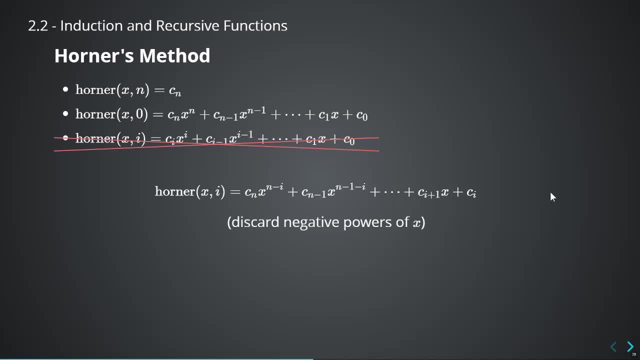 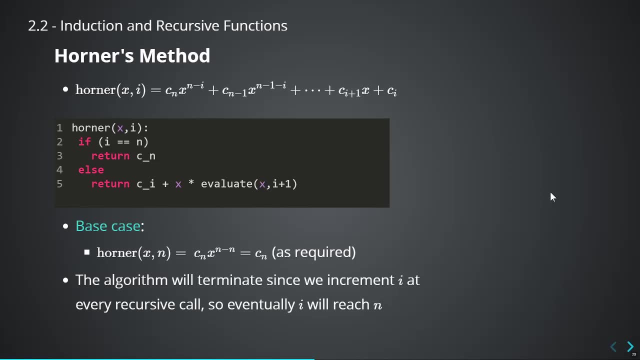 induction again, and the trickiest bit is to find that actual statement. but because when we once we have the statement, so i'm writing up here once you have the statement, uh, the base case is simple, right, the base case. uh, you can see that the base case is when i equal to n. 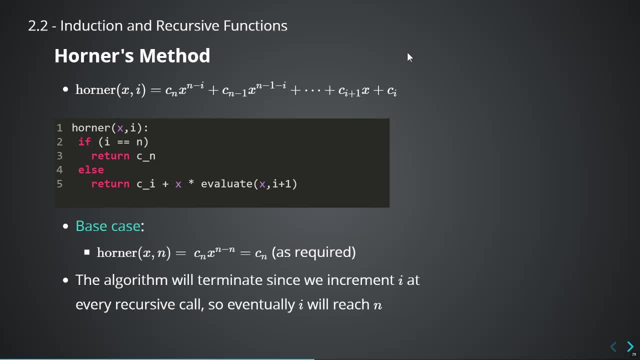 and it goes like just before: um, just as before. just assume we have a same input for i, so i is going to be between 0 and n. well, actually, in this case we always think about how it's going to be n, because we want to evaluate a polynomial size. 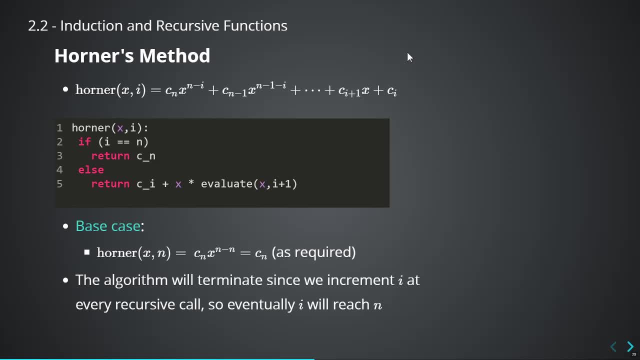 n, oh sorry, of degree n. so the base case there is horner x, n and it's going to give us cn, which is, which means that the statement up here is correct. now is this algorithm going to terminate? yeah, it will, because if we start at i, equal to 0. 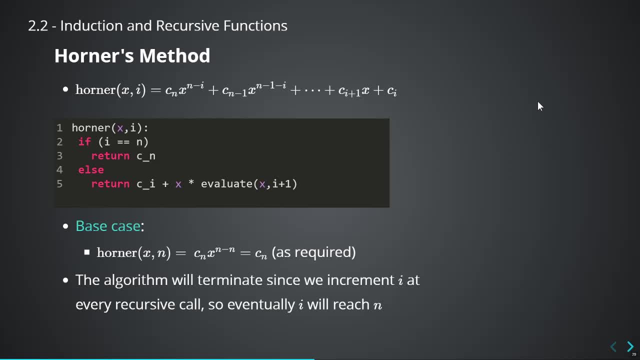 we are. we're going to be increasing i plus um. we're going to be increasing i every time we make a recursive call, so i becomes i plus 1, i plus 2 and so on. eventually it will reach n, in which case the algorithm will terminate. 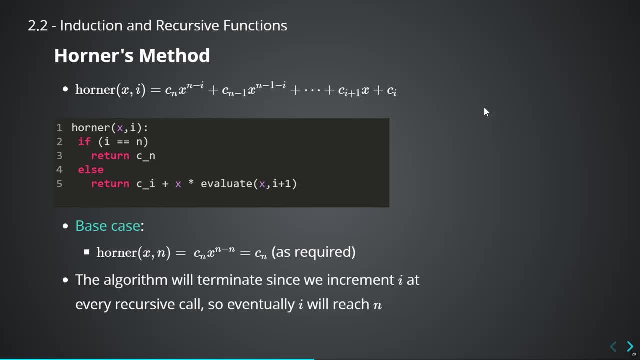 so, yes, it will terminate. the base case is correct. um, good, we're good to go. moving on to the induction step. uh, what is the hypothesis? just a statement, not there, but put in k instead of i, and you're done. that's your induction hypothesis. and finally, we got to show. 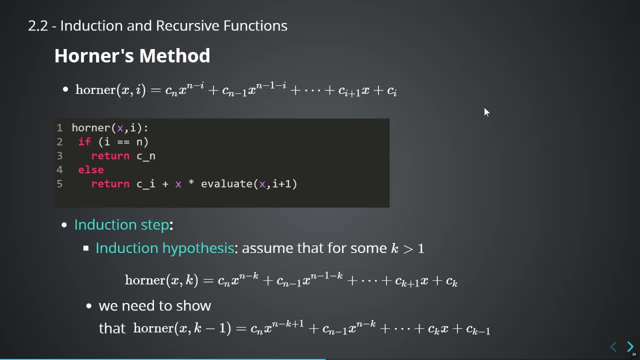 that. um, the next step: like we assume that horner x k is correct, then we have to show that horner x k minus 1 is also correct. now, not k plus 1, it's actually k minus 1. why? because we keep on uh, increasing. i right as. 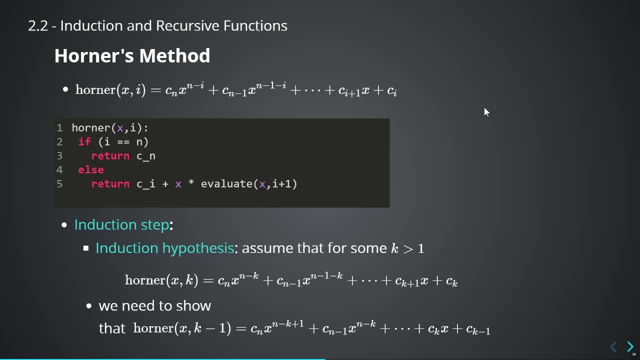 we go so. so what happened is um before we? we say that, oh, if it's true for one, then it's going to be, then two is going to be true as well. if two is true, then three is going to be true as well. now we're flipping that. now we're, now we're. 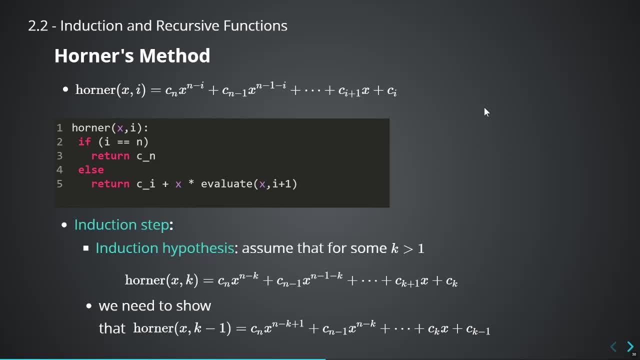 saying that: oh, if it was true for n, then it would be true for n minus one as well. if it's true for five, then it'd be true for four. why? because the end goal is: you want to show that this is correct, for i equal to zero. 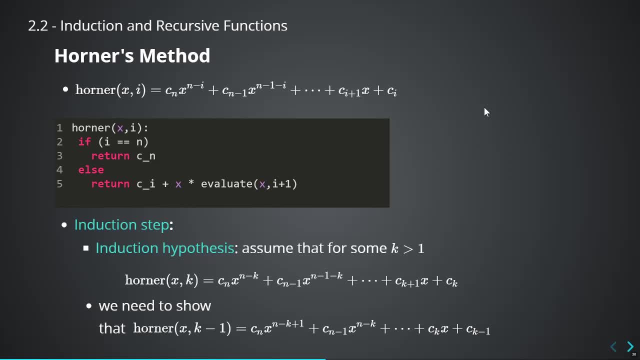 all right. so we have to do the other way around, and to actually do that is pretty simple. um, it's just, there's only one line there, right, just only line five. that's the way we actually do any work. so if i call horner x k. 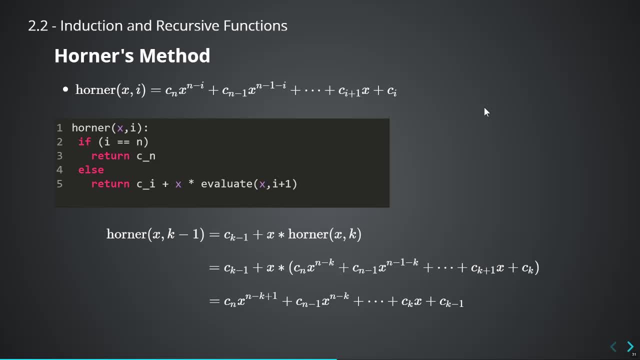 minus one. um, you're going to use horner x k and let's just assume horner x k is correct, so i'll get this polynomial here in the brackets. um, sorry, i can't help. yep, that, that one there. assuming that is correct, i'm going to 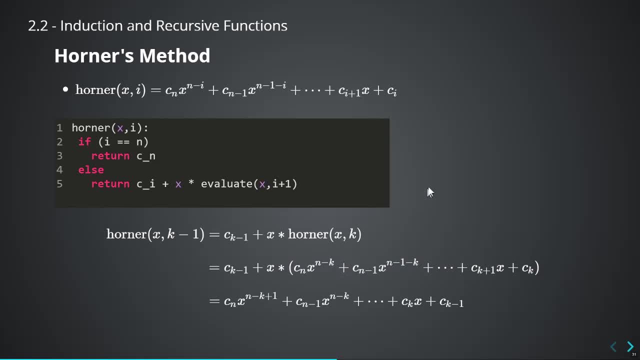 multiply by x. that's line five. and then i'm going to add ci to it, i'm going to add c, k minus one to it, and when i do that i will end up with the polynomial um. well, the last line there. sorry, again, it's hard to. 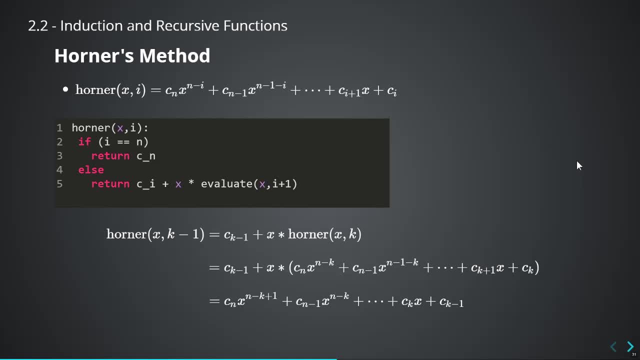 read this. um, it's hard to read this, uh, on the lecture, but, um, if you just sit down and write this down or you can see it on a slide, um, hopefully you think that this is correct, okay, so yeah, it's actually simple to show that the inductive relationship. 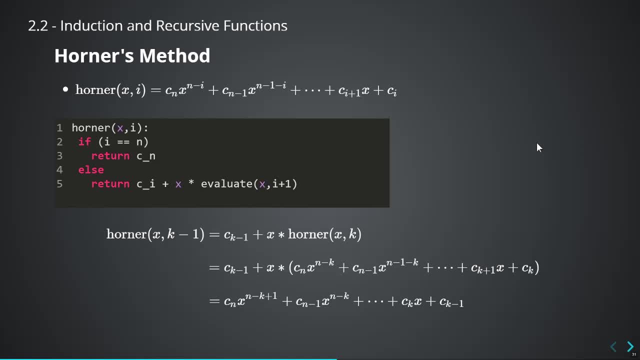 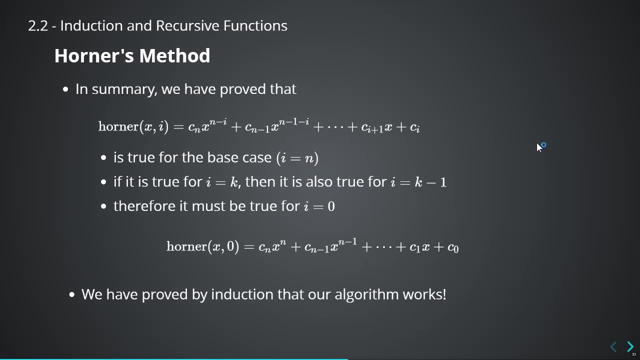 this is simple to show that um, if it's true for horner x k, then it's also true for horner x k minus one. so again, in summary, this is induction um. we have the statement that we want to prove to be true, right and um with the goal is we want to show 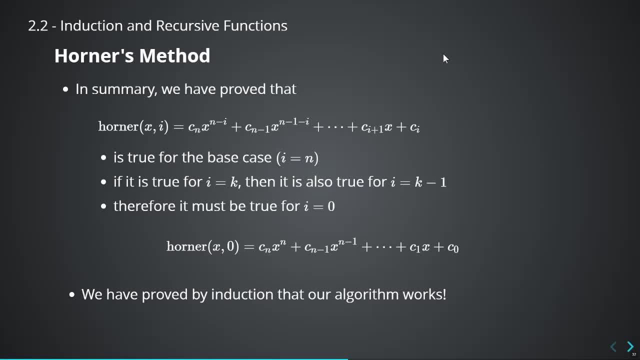 that this is true for i equal to zero, and we show that this is true for the base case. we show that the statement is true for i equal to n, the function works for i equal to n and we also argue that if it's true for i equal to, 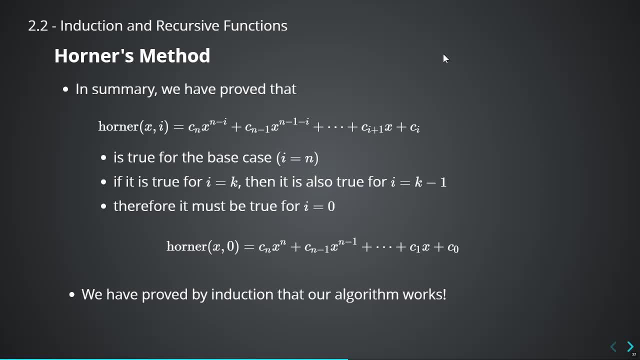 k, then it's also true for i: equal to k minus one. so it must be true for i: equal to zero. you know, because it's true for five, it's true for four, it's true for four, it's true for three, and so on until we get to zero. 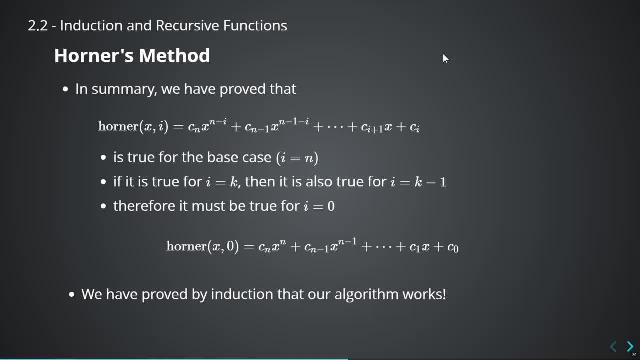 we have shown by induction that our algorithm works. it does compute f to the x, sorry, um, it does compute fx because if i have horner x zero, then from the uh, from what i have up here, from the formula, you can see that horner x zero gives you the whole.